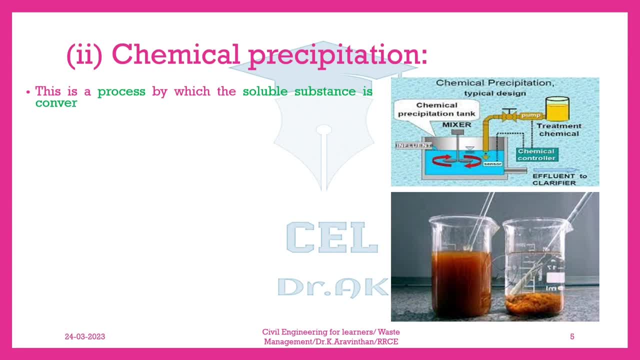 This is a process by which the soluble substance is converted to an insoluble form, either by a chemical reaction or by a change in the composition of the solvent to diminish the solubility of the substance in it. Settling and or filtration can then remove the precipitated solids. 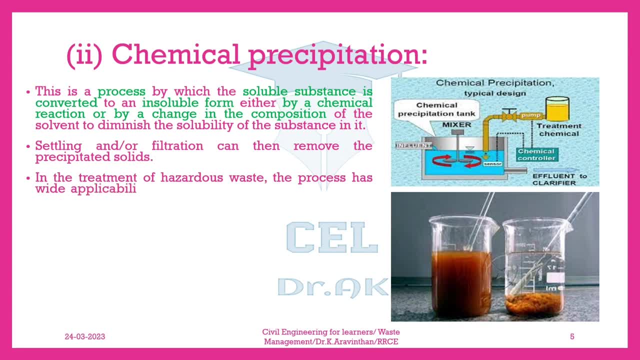 In a treatment of hazardous waste. the process has wide applicability in the removal of toxic metals from aqueous wastes by converting them to an insoluble form. This includes wastes containing arsenic, barium, cadmium, chromium, copper, lead, mercury, nickel, selenium, silver, thallium. 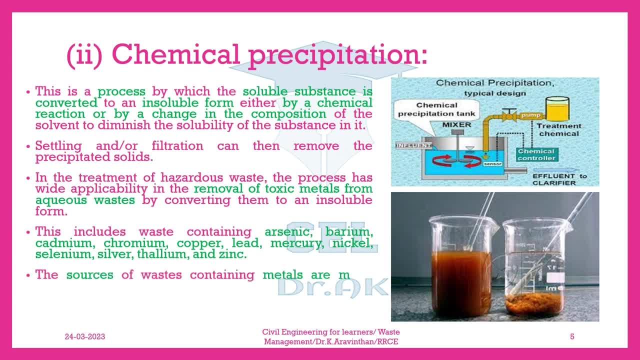 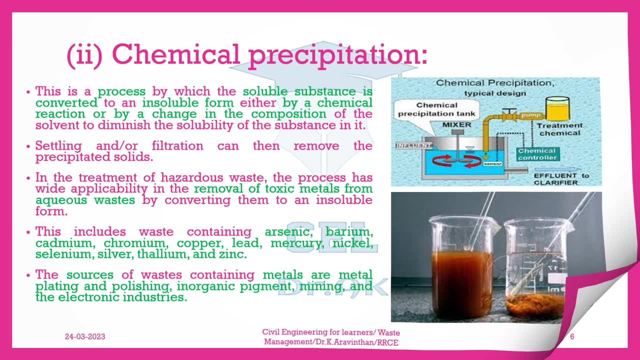 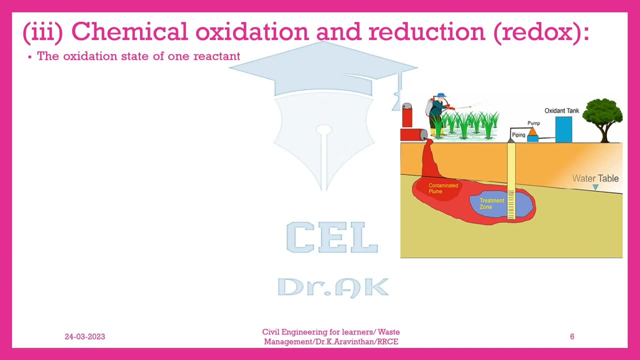 and zinc. The sources of waste-containing metals are metal plating and polishing, inorganic pigment mining and the electronic industries. 3. Chemical oxidation and reduction. The oxidation state of one reactant is raised, while that of the other reactant is lowered When electrons are removed from an ion. 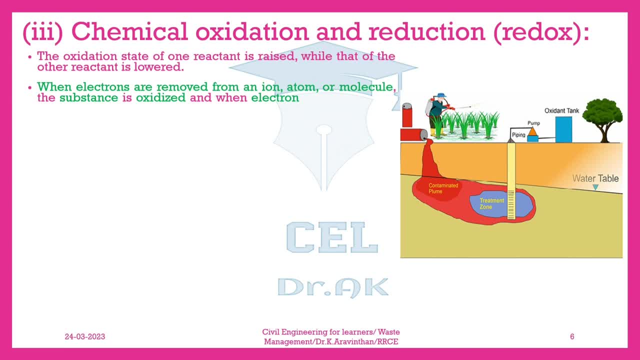 atom or molecule, the substance is oxidized, and when electrons are added to a substance, it is reduced. Such reactions are used in the treatment of metal-bearing wastes, sulfides, cyanides and chromium, and in the treatment of many organic wastes such as phenols. 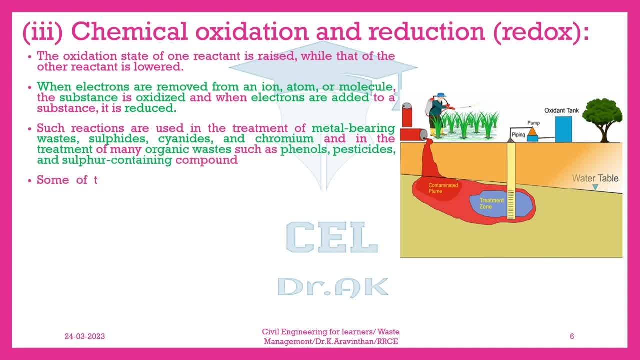 pesticides and sulfur-containing compounds. Some of the commonly used oxidizing agents are sodium hypochlorite, hydrogen peroxide, calcium hypochlorite, potassium permanganate and ozone. Reducing agents are used to treat wastes containing hexavalent chromium, mercury, organometallic compounds and chelated metals. 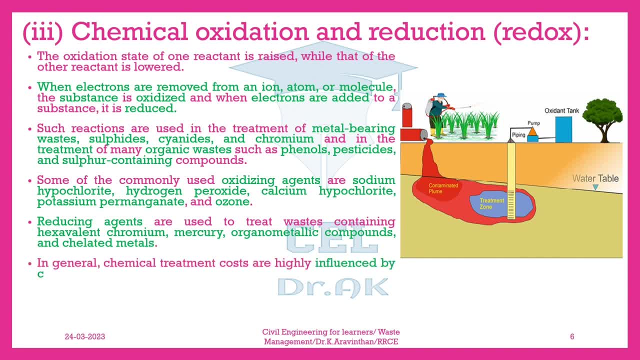 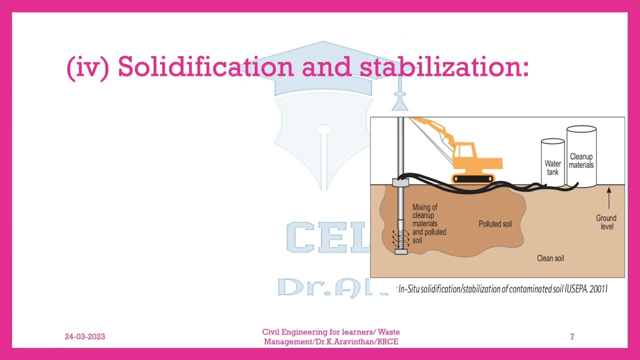 In general, chemical treatment costs are highly influenced by chemical costs. This oxidation and reduction treatment tends to be more suitable for low concentration in wastes. 4. Oxidation and reduction of wastes and chemicals in the treatment of metal-bearing wastes. 4. Solidification and stabilization. 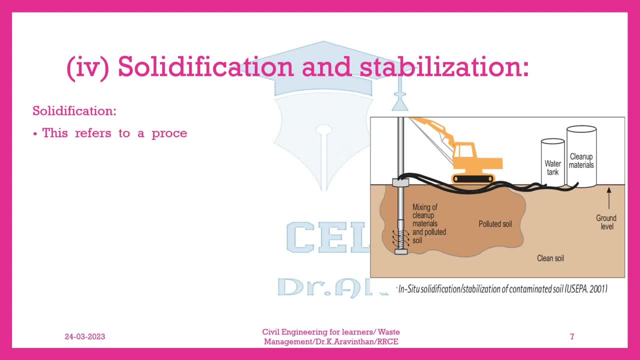 Solidification: This refers to a process in which materials are added to the waste to produce a solid. It may or may not involve a chemical bonding between the toxic contaminant and the additive. Stabilization: This refers to a process by which waste is converted to a more chemically. 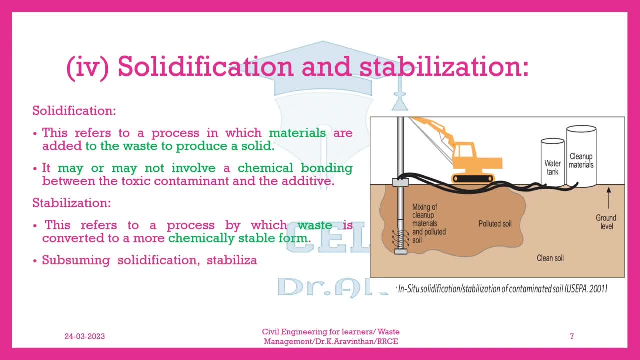 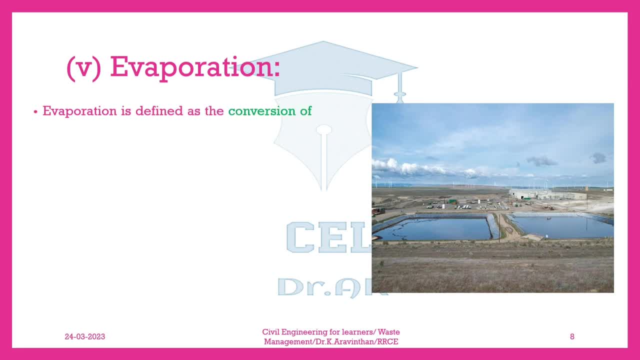 Evaporation. Evaporation is defined as the conversion of a liquid from a solution or slurry into vapor. Evaporation is used in the treatment of hazardous waste, and the process equipment is quite flexible and can handle waste in various forms: aqueous slurries. 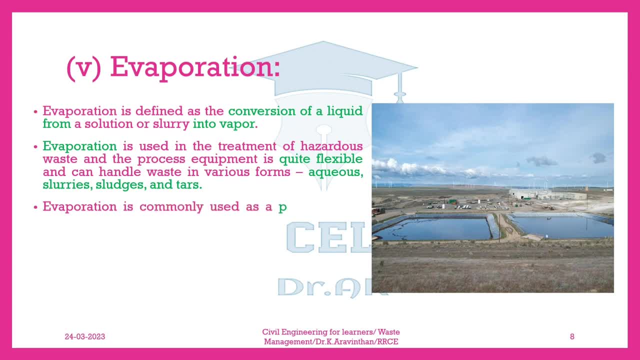 sludges and tars. Evaporation is commonly used as a pre-treatment method to decrease quantities of material for final treatment. It is also used in cases where no other treatment method was found to be practical, such as in the concentration of trinitrotoluene TNT. 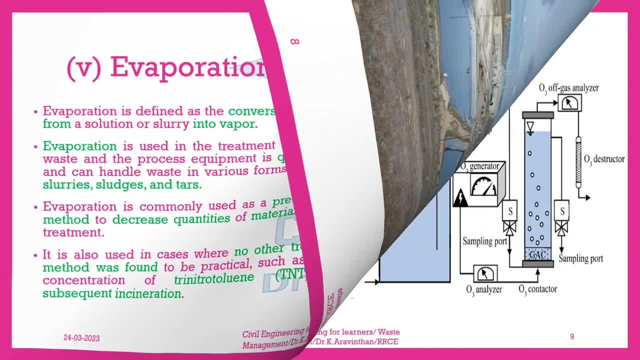 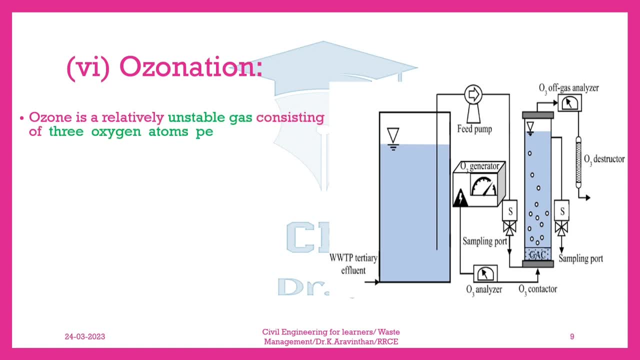 for subsequent incineration. 6. Ozonation: Ozone is a relatively unstable gas consisting of three oxygen atoms per molecule- O3, and is one of the strongest oxidizing agents known. It can be substituted for conventional oxidants such as chlorine, hydrogen peroxide and potassium permanganate, Ozone and UV radiations. 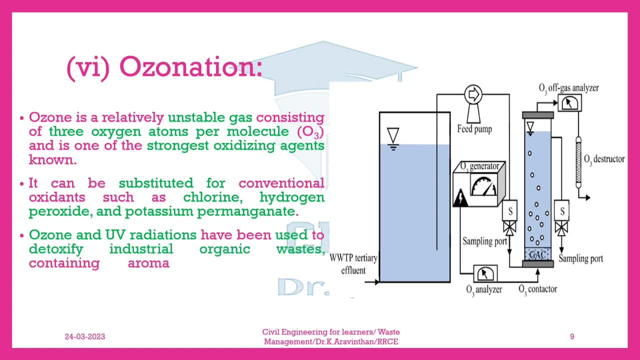 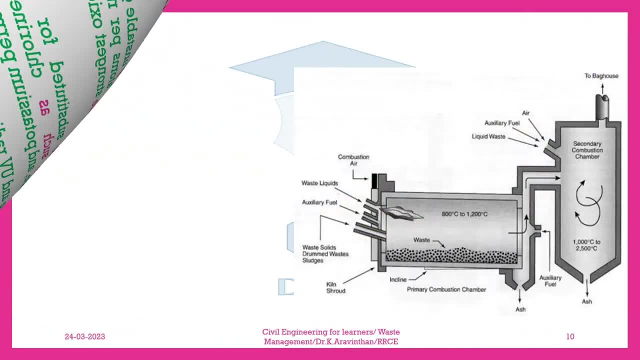 have been used to control the concentration of oxygen atoms per molecule O3, and is one of the to detoxify industrial organic wastes containing aromatic and aliphatic polychlorinated compounds, ketones and alcohols. 2. Thermal Treatment. 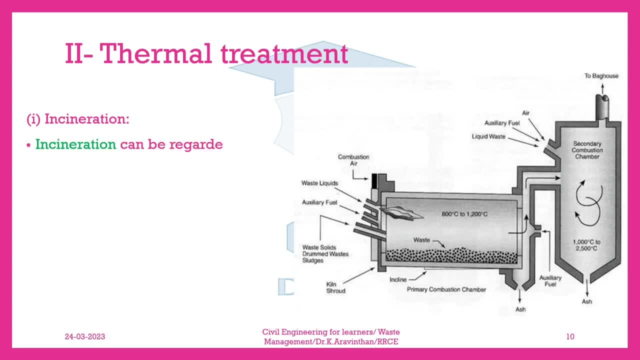 1. Incineration. Incineration can be regarded as either a pre-treatment of hazardous waste prior to final disposal, or as a means of valorizing waste by recovering energy. It includes both the burning of mixed solid waste or the burning of selected parts of the 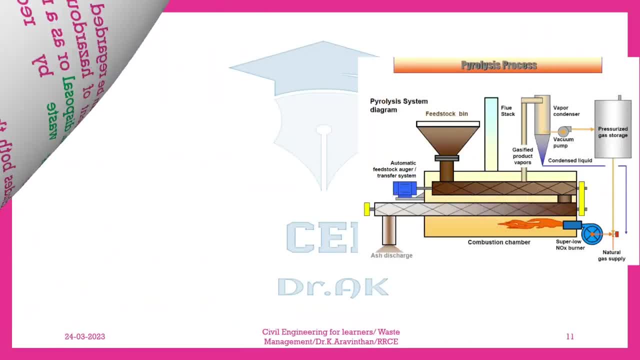 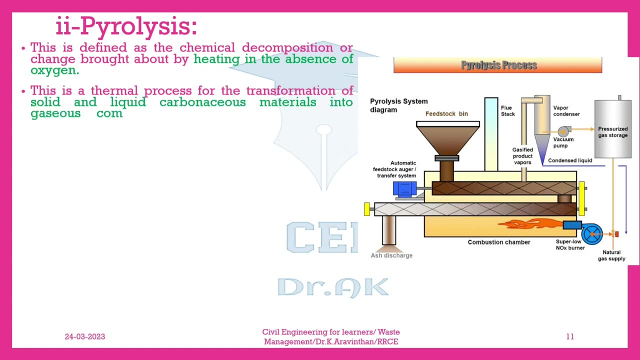 waste stream as a fuel. 2. Rholysis: This is defined as the chemical decomposition or change brought about by heating in the absence of oxygen. This is a thermal process for the transformation of solid and liquid carbonaceous materials into gaseous components and the solid residue containing 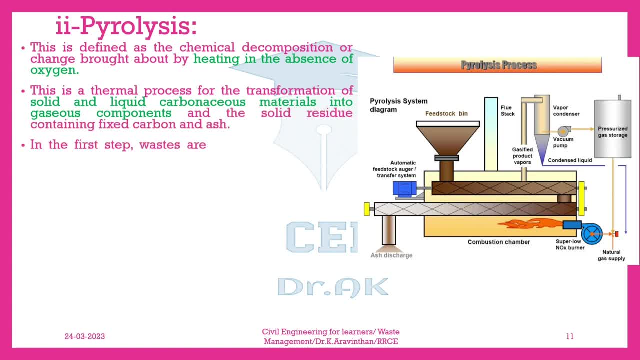 fixed carbon and ash. In the first step, wastes are heated, separating the volatile contents- example: combustible gases, water vapor, etc. from non-volatile char and ash. In the second step, volatile components are burned under proper conditions to assure the incineration of all. 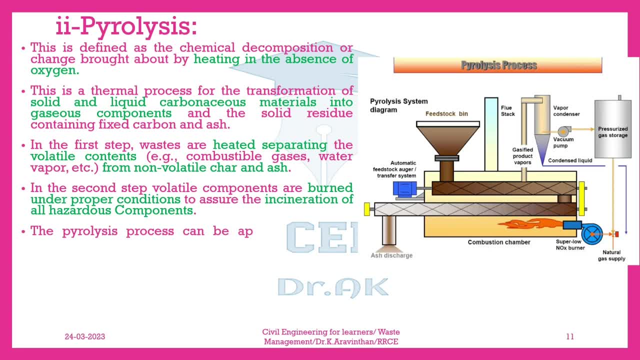 hazardous components. The pyrolysis process can be applied to solids, plastic sludges and liquid wastes. Materials containing salts and metals which melt and volatilize at normal incineration temperatures, Materials like sodium chloride, NaCl, zinc, Zn and lead, Pb. when. 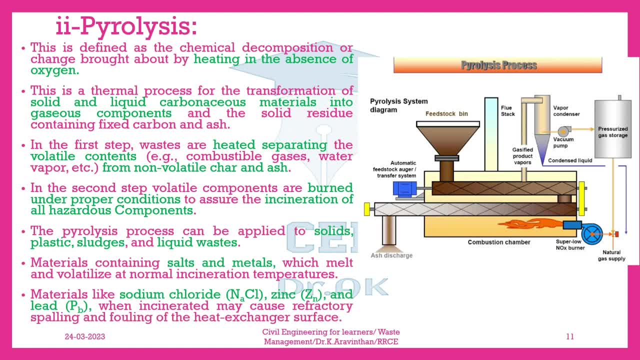 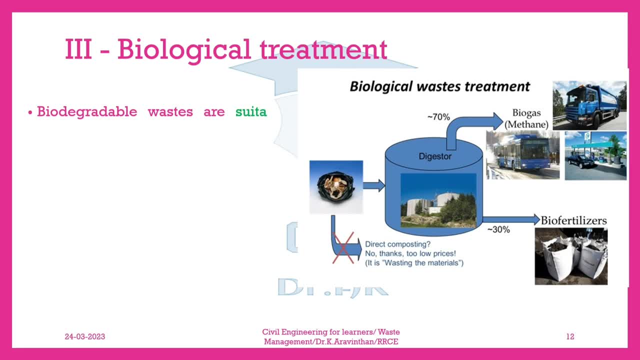 incinerated may cause refractory spalling and fouling of the heat exchanger surface. 3. Biological Treatment: Biodegradable wastes are suitable for land treatment, Radioactive wastes, highly volatile reactive flammable liquids and inorganic wastes such as. 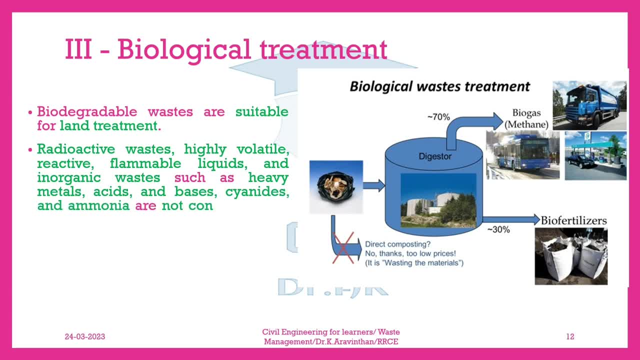 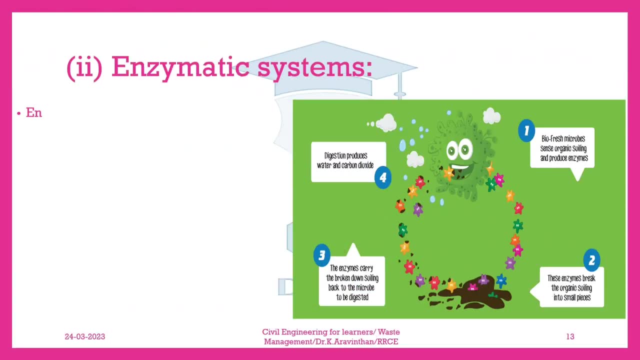 heavy metals, acids and bases, cyanides and ammonia are not considered for land treatment. Land treatability of organic compounds often follows a predictable pattern for similar types of compounds. 2. Enzymatic Systems: Enzymes capable of transforming hazardous waste chemicals into non-toxic products can. 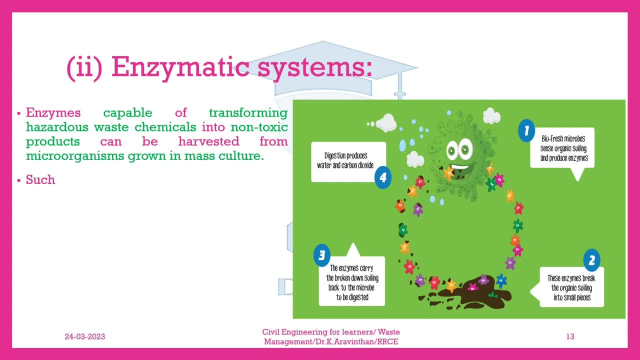 be harvested from microorganisms grown in mass culture. Such crude enzyme extracts derived from microorganisms have been shown to convert pesticides into less toxic and persistent products. The factors of moisture, temperature, aeration, soil structure, organic matter content, seasonal variation and the availability of soil nutrients influence the presence and abundance of. 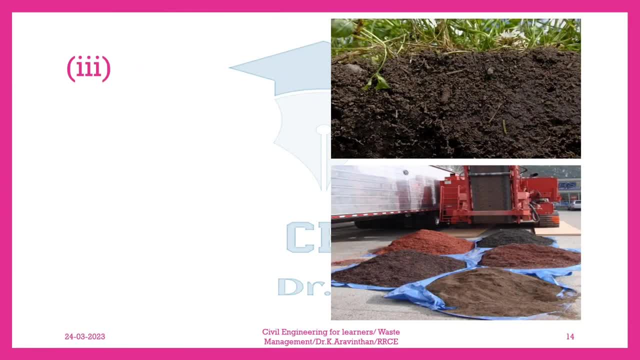 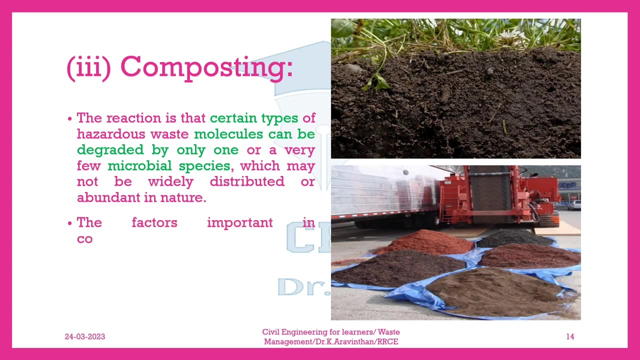 enzymes. 3. Composting: The reaction is that certain types of hazardous waste molecules can be degraded by only one or a very few microbial species, which may not be widely distributed or abundant in nature. The factors important in composting hazardous wastes are those that govern all 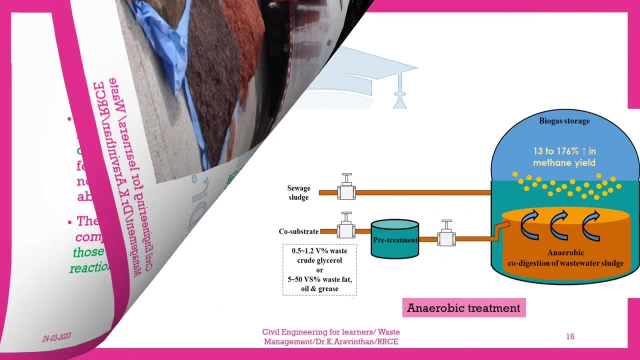 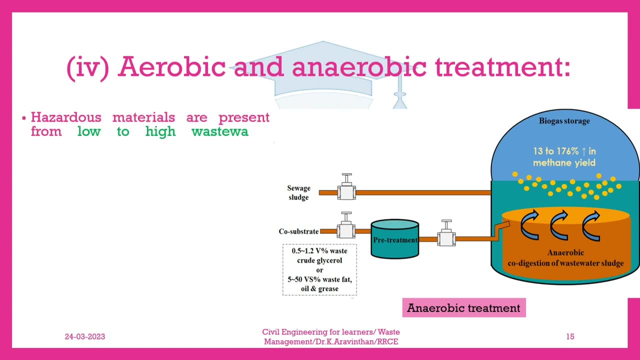 biological reactions. 4. Aerobic and Anaerobic Treatment. Hazardous materials are present from low to high wastewater, leachate and soil concentrations. These wastes are characterized by high organic content, low and high pH, elevated salt levels sometimes.